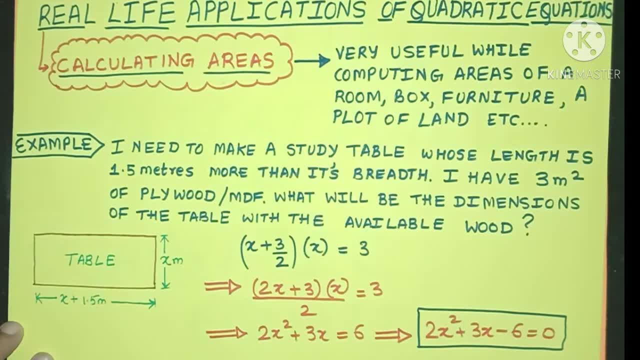 furniture, maybe a piece of land, a garden, etc. So I've just given here an example. So suppose I want to make a study table, friends, where the length has to be, say, 1.5 meters more than the breadth, Okay, And suppose I have three meters square of wood with me. So what will be the dimensions of the table if I want to make it with the available area of wood? So, friends, in this case we'll use the area of 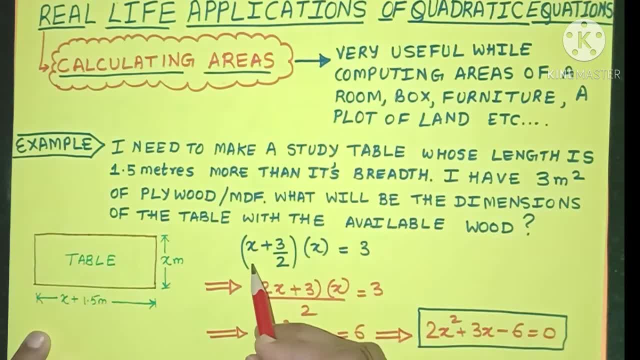 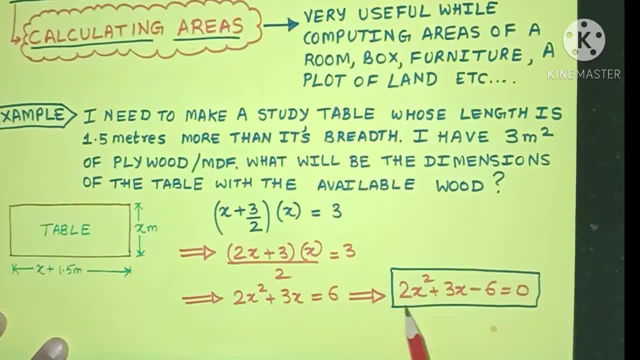 the table formula, the area of a rectangle. So you will see that I have used that formula over here And we have simplified and got a quadratic equation. On solving this quadratic equation, you will come to know what will be the value of the breadth, So that with three meters square of wood you can create this table such that the length is also 1.5 meters more than the breadth. So in those situations, friends, where a variable is, 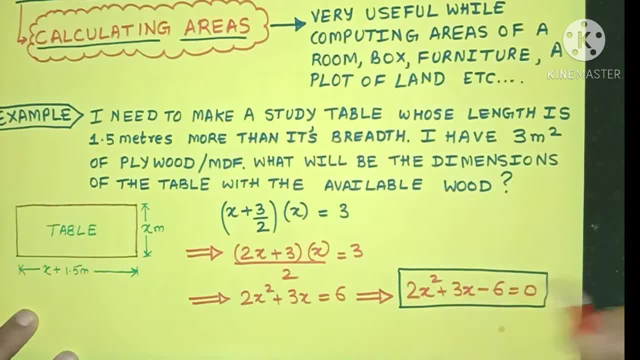 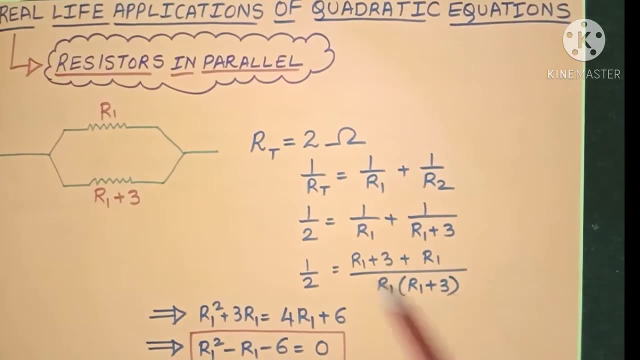 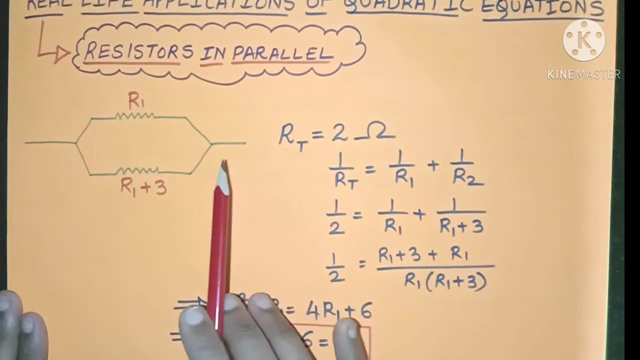 simplified with itself and we get the square of the variable. quadratic equations always come into play. So quadratic equations are very useful in calculating areas. Now let's go to the next application of quadratic equations, And that is in physics, friends. that is when we talk about parallel resistors. So, as you can see here, here is a very simple circuit of two resistors which are in parallel, And suppose I want the total resistance. to be two ohms, right. So here is our formula for resistors in parallel. we know the total resistance as two ohms, And one resistance is always supposed three ohms or two ohms more than the other resistor. So I just need to substitute these values, friends, and you will observe that we end up getting a quadratic equation in R One. So, once again, wherever a variable is multiplied with itself, you will always end up getting a quadratic equation, And so the total resistance is always, suppose, three ohms. 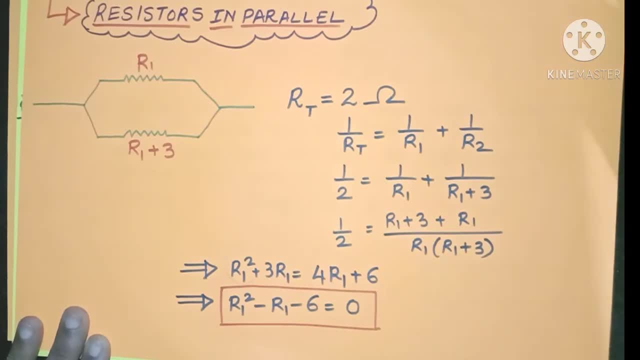 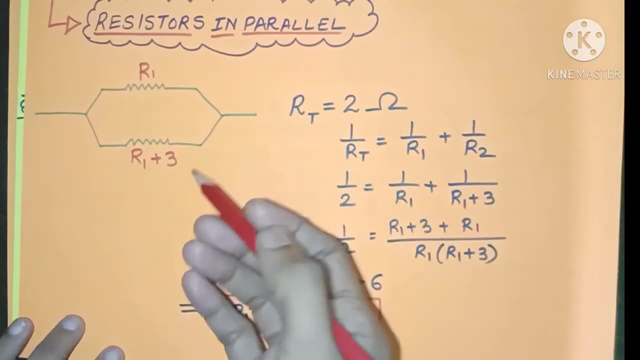 getting a quadratic equation which, when solved, you will come to know what value of resistance has to be applied in this circuit to get this desired total resistance of 2 ohms. So quadratic equations is very useful in these situations where we have resistors in parallel. 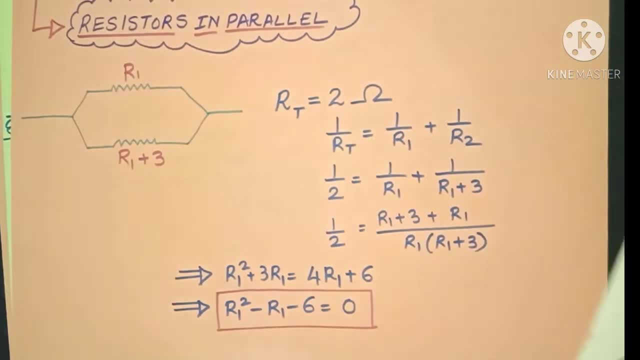 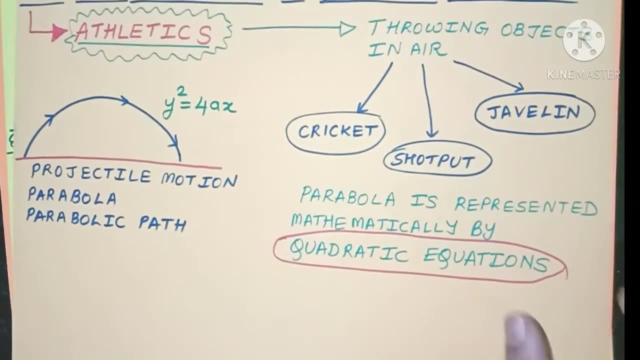 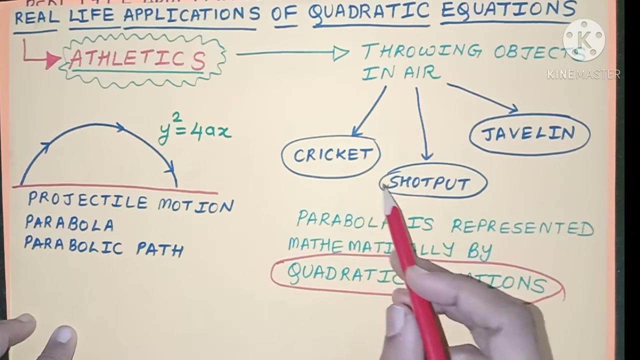 Now let's go to the next application. So, friends, the next application of quadratic equations is, yes, athletics. So athletics can't be far behind, and quadratic equations is used a lot in athletics. Now I'll tell you how. So in games like cricket, shot, put javelin throw, we have objects being thrown in air. 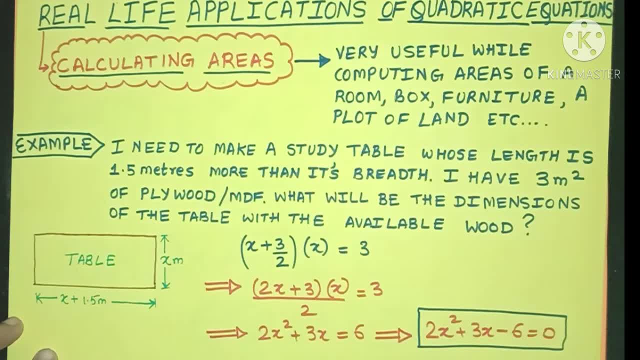 than the breadth. Okay, and suppose I have three meters square of wood with me. So what will be the dimensions of the table if I want to make it with the available area of wood? So, friends, in this case we'll use the area of the table formula, the area of a rectangle. So you will see that I have used that. 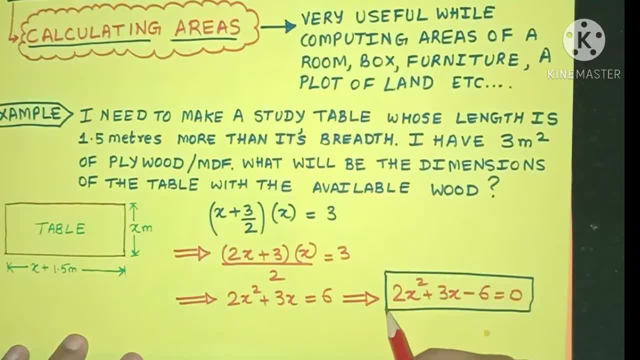 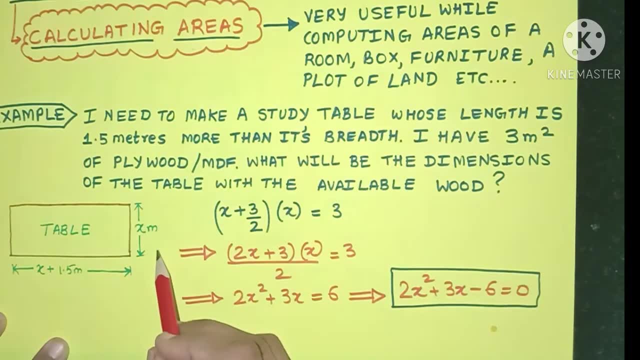 formula over here and we have simplified and got a quadratic equation. On solving this quadratic equation, you will come to know what will be the value of the breadth, so that with three meters square of wood you can create this table such that the length is also 1.5 meters more than the 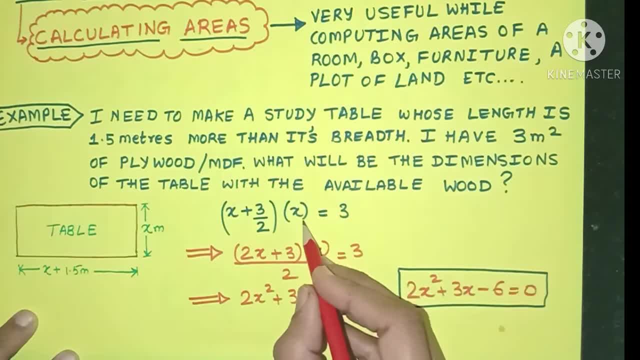 breadth. So in those situations, friends, where a variable is multiplied with itself and we get the square of the variable, quadratic equations always come into play. So quadratic equations are very useful in calculating areas. Now let's go to the next application of quadratic equations. 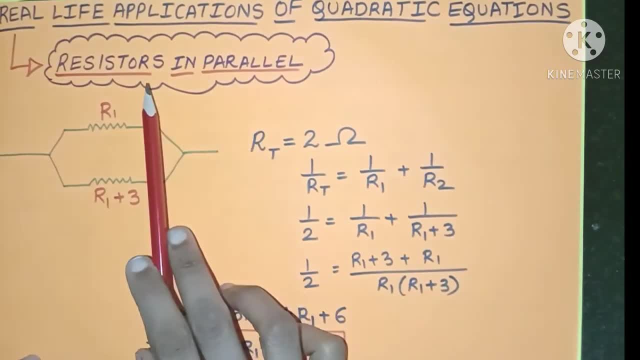 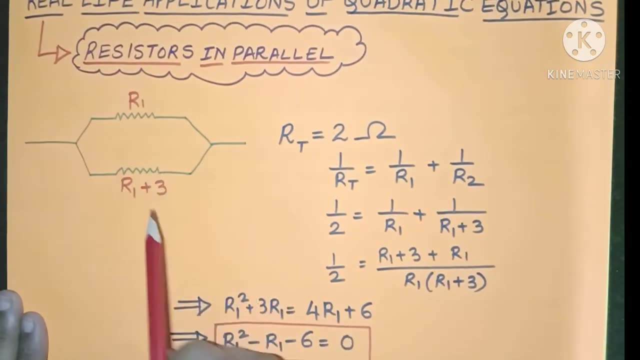 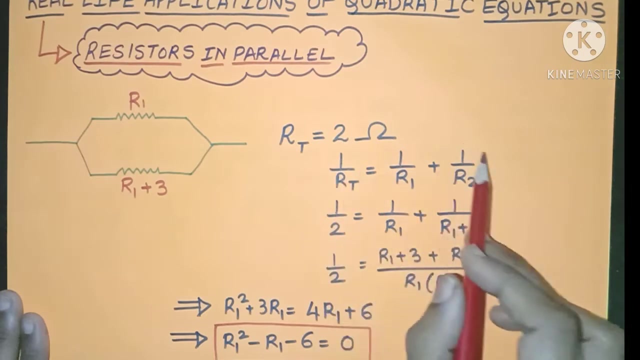 and that is in physics, friends, that is, when we talk about parallel resistors. So, as you can see here, here is a very simple circuit of two resistors which are in parallel, and suppose I want want the total resistance to be 2 ohms, right? So here is our formula for resistors in parallel. 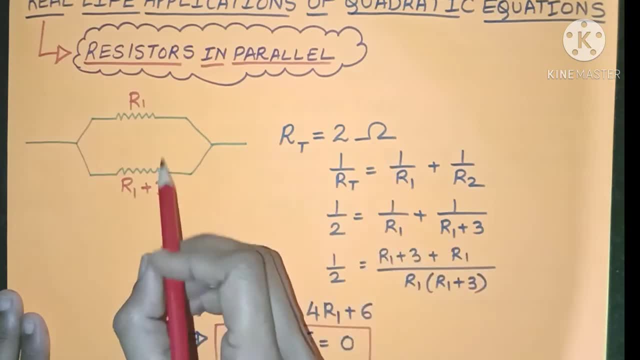 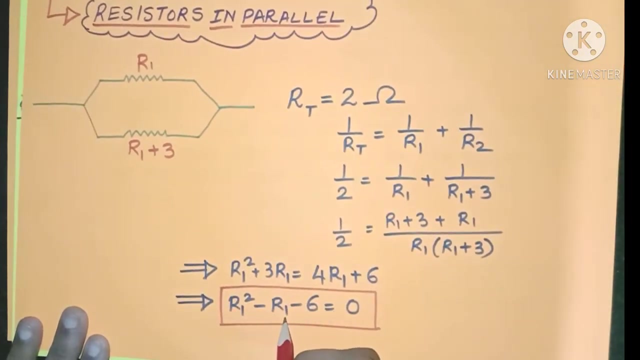 We know the total resistance as 2 ohms, and one resistance is always, suppose, 3 ohms or 2 ohms more than the other resistor. So I just need to substitute these values, friends, and you will observe that we end up getting a quadratic equation in R1.. So, once again, wherever a variable 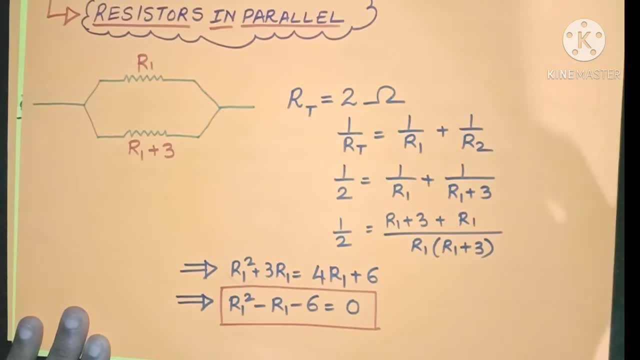 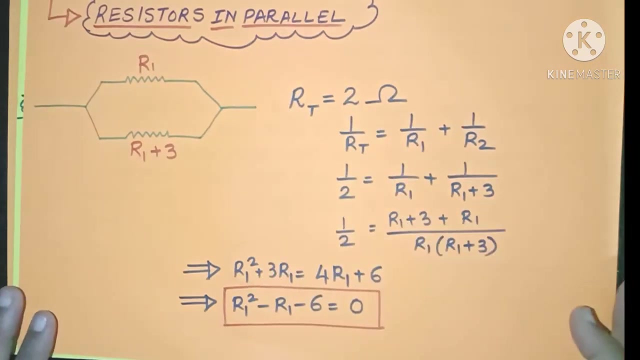 is multiplied with itself, you will always end up getting a quadratic equation which, when solved, you will come to know what value of resistance has to be applied in this circuit to get this desired total resistance of 2 ohms. So quadratic equations is very useful in these situations. 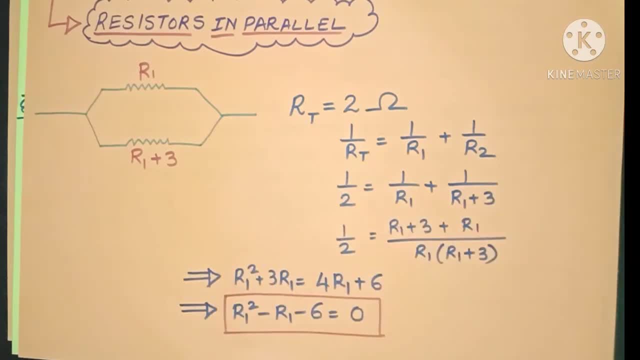 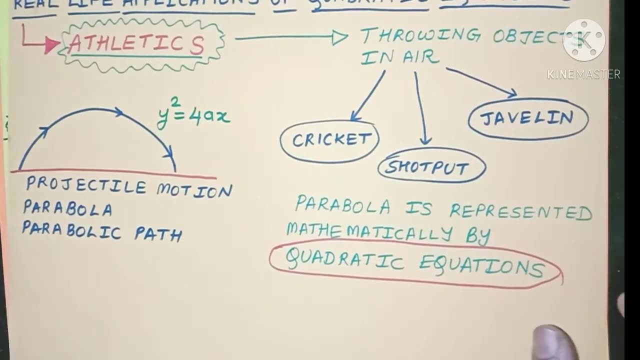 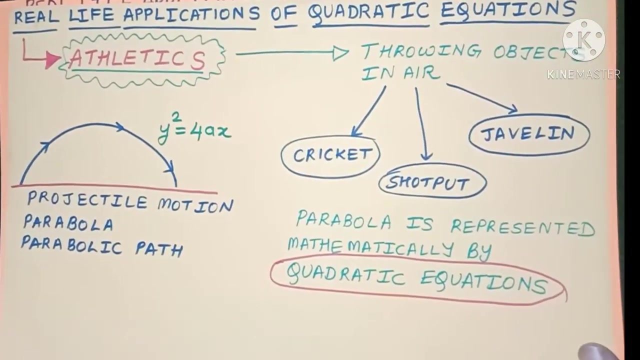 where we have resistors in parallel. Now let's go to the next application. So, friends, the next application of quadratic equations is, yes, It's athletics. So athletics can't be far behind, and quadratic equations is used a lot in athletics. Now I'll tell you how. So in games like cricket, shot, put, javelin throw. we have. 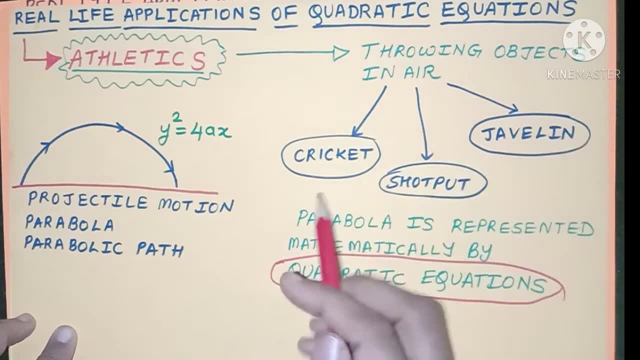 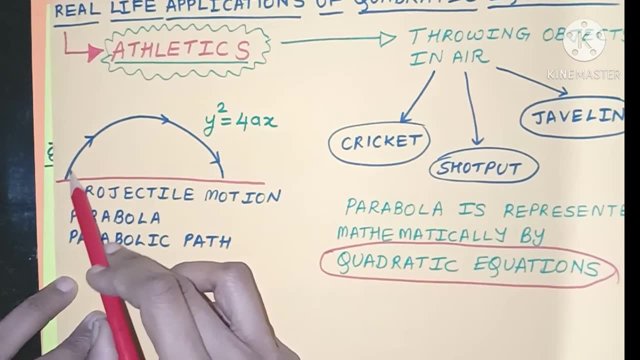 objects being thrown in air. So you have a ball which is being thrown in the air, or a javelin which is being thrown in the air. So all these objects, when moving in the air, friends, they always follow this particular type of motion. If you see, this is. 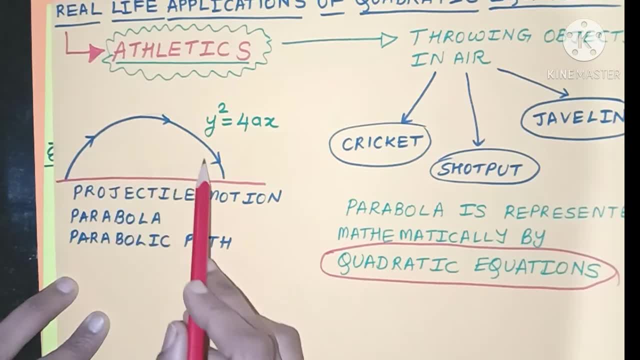 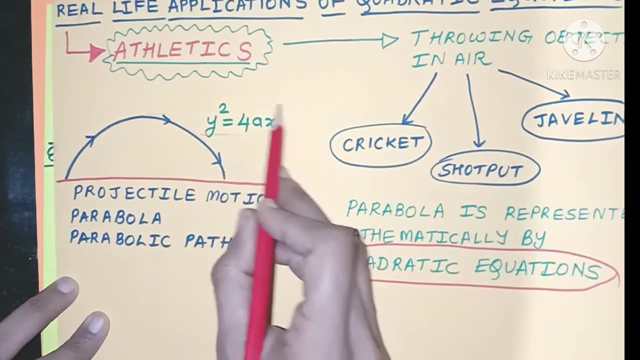 called a projectile motion and this shape of the curve that is formed is called a parabola. friends, What is it called A parabola? and we say that this is a parabolic path and always, a parabola is represented by a quadratic equation: y square equal to 4a- x. So whenever we have 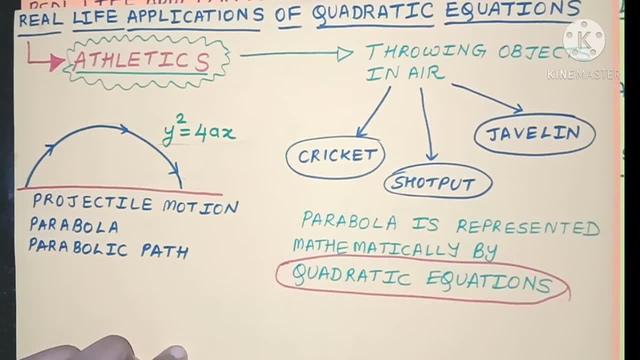 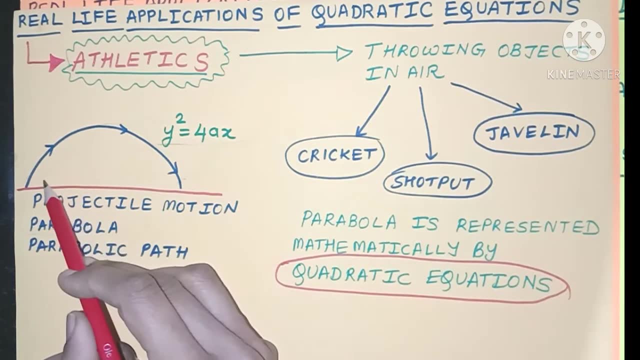 analysis of such games, where you know a bowler is throwing a ball or an athlete is throwing a ball- the javelin- they always follow this particular parabolic path, which can be represented mathematically by quadratic equations. So quadratic equations are used a lot. if you want to. 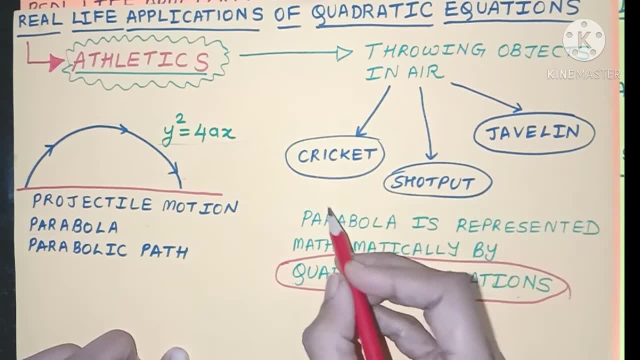 estimate at what speed should a ball, you know, leave the bat so that you get a boundary, or what should be the speed with which an athlete should throw a javelin so that it reaches a particular maximum height or it reaches the farthest distance. So, for all this analysis, quadratic equations always come into play and they are very 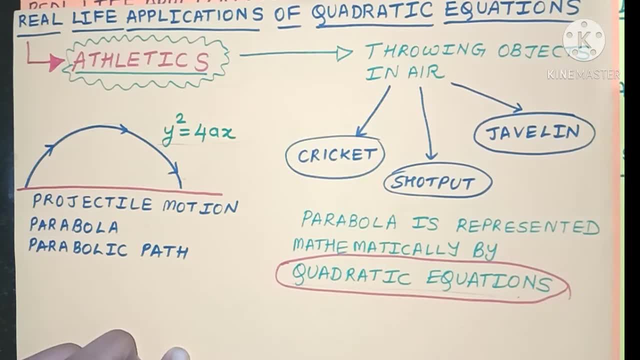 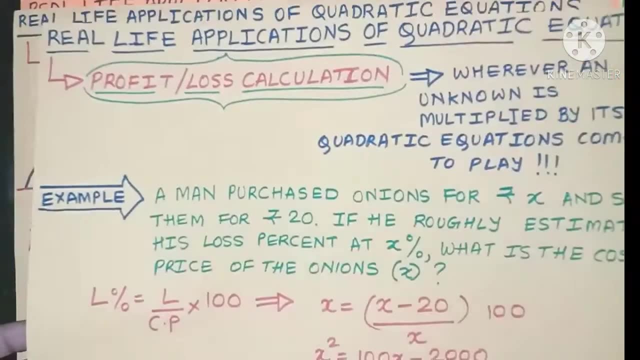 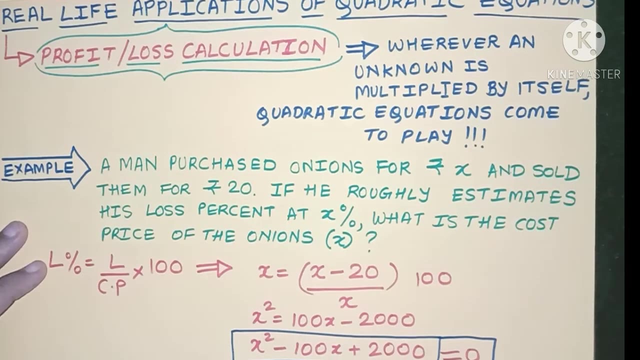 useful. So quadratic equations is used a lot in athletics. Now, coming to the next real life application of quadratic equations, we have profit and loss calculation friends. So again the same concept: whenever an unknown is multiplied by itself, you will get a quadratic equation. So 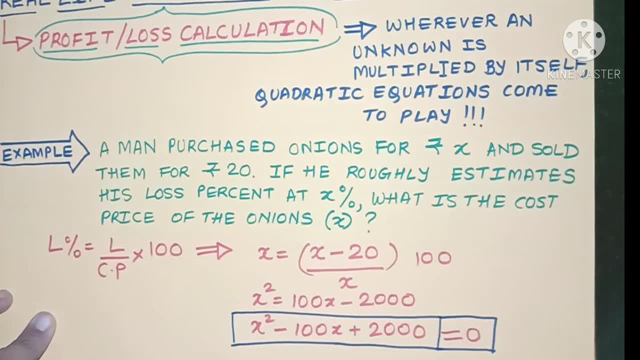 here is an example. So suppose a man has purchased onions, say for X amount of rupees, and he sold them for 20 rupees. Now he has incurred a loss and he roughly estimates that his loss percent is, say, X percent. Now what will be the cost price of the? 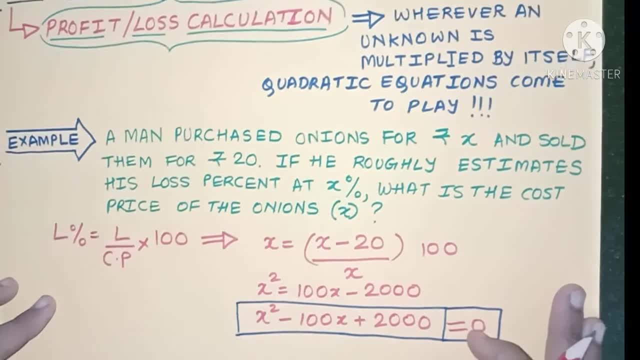 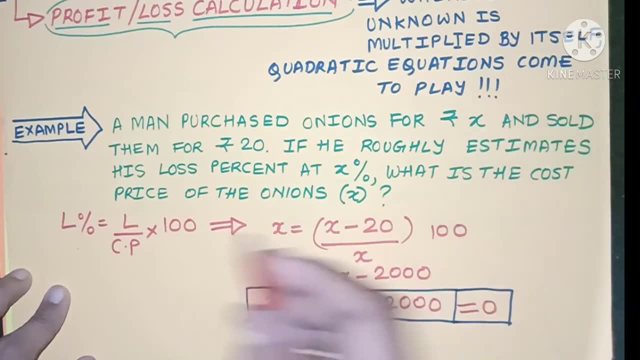 onions. So this can be solved very easily with quadratic equations. So, as you know the formula for loss percent, or you know, in case he gets a profit, you can substitute the profit percent formula also. So you just need to substitute the values which are there and you will again end up getting a. 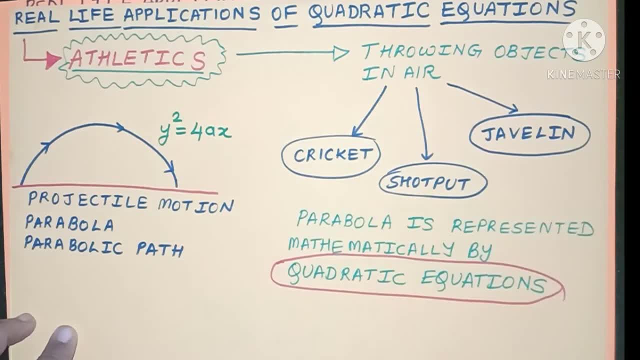 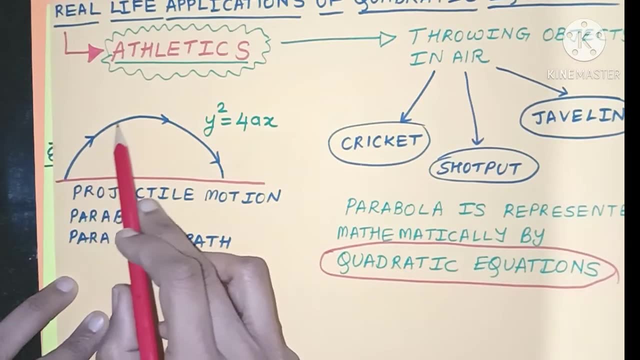 So you have a ball which is being thrown in the air, or a javelin which is being thrown in the air. So all these objects, when moving in the air, friends, they always follow this particular type of motion. If you see, this is called a projectile. 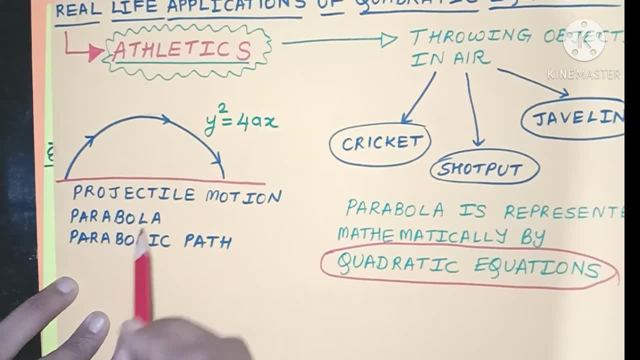 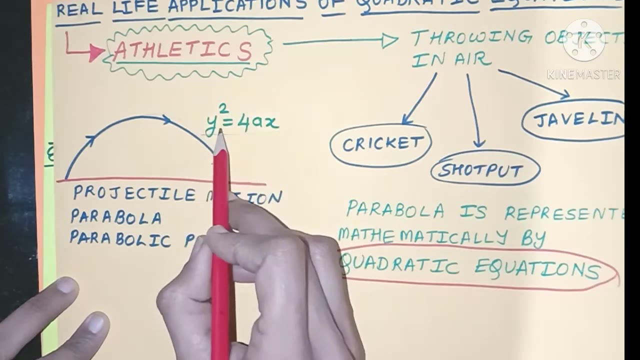 This is a projectile motion and this shape of the curve that is formed is called a parabola. friends, What is it called A parabola? and we say that this is a parabolic path and always, a parabola is represented by a quadratic equation: y square equal to 4ax. 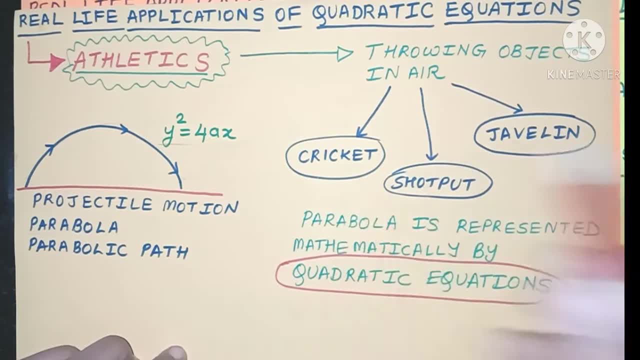 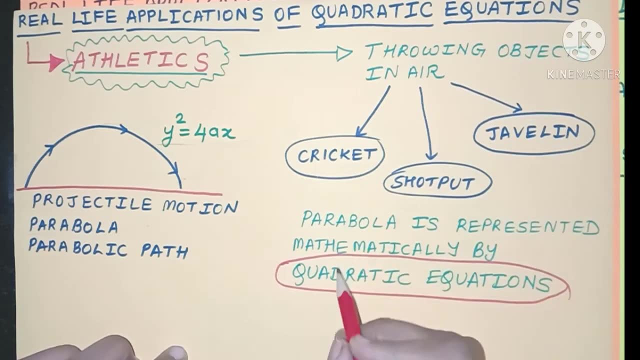 So whenever we have analysis of such games, where you know a bowler is throwing a ball or an athlete is throwing the javelin, They always follow this particular parabolic path which can be represented mathematically by quadratic equations. So quadratic equations are used a lot if you want to estimate at what speed should a ball. 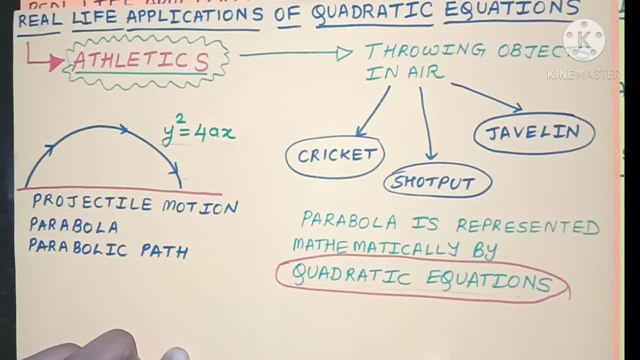 you know, leave the bat so that you get a boundary, or what should be the speed with which an athlete should throw a javelin so that it reaches a particular maximum height or it reaches the farthest distance. Okay, So for all this analysis, quadratic equations always come into play, and they are very useful. 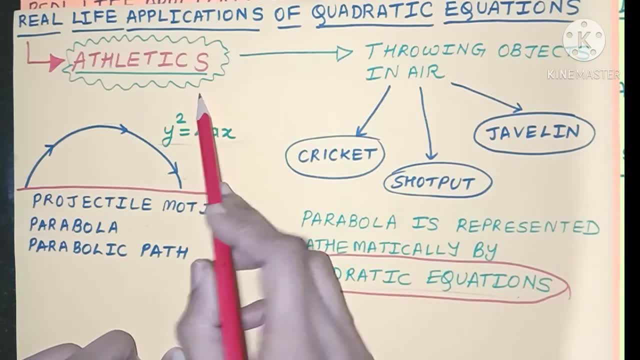 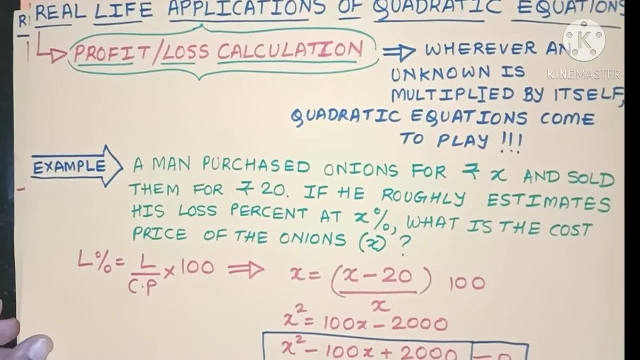 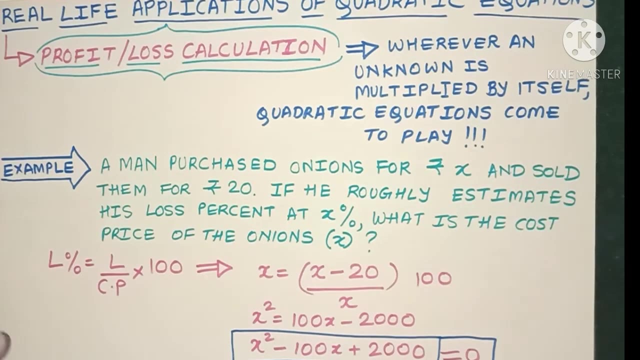 So quadratic equations is used a lot in athletics. Now, coming to the next real life application of quadratic equations, we have profit and loss calculation friends. So again the same concept: whenever an unknown is multiplied by itself, you will get a quadratic equation. So here is an example. 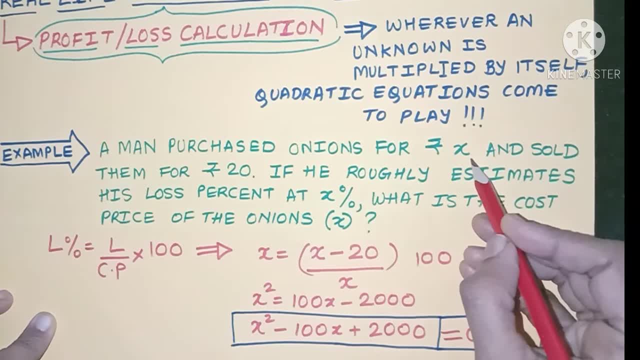 So suppose a man has purchased Onions, say for X amount of rupees, and he sold them for 20 rupees. Now he has incurred a loss and he roughly estimates that his loss percent is, say, X percent. Now what will be the cost price of the onions? 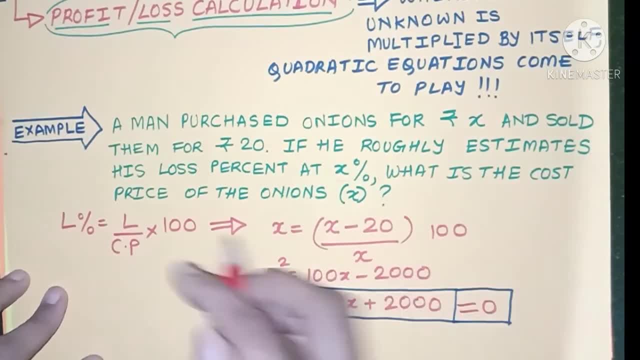 So this can be solved very easily with quadratic equations. So, as you know the formula for loss percent, or you know, in case he gets a profit you can substitute the profit percent formula also. So loss percent is loss upon cost price into 100.. So you just need to substitute the values which are there and you will again end up. 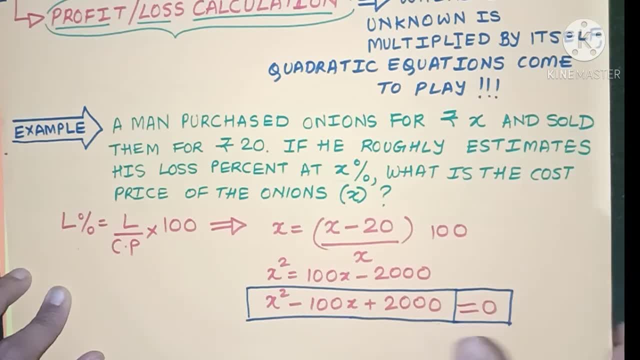 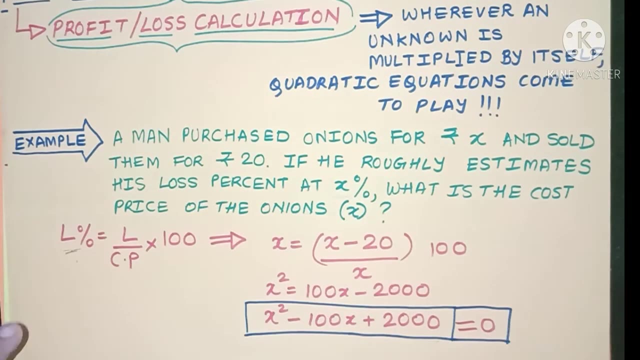 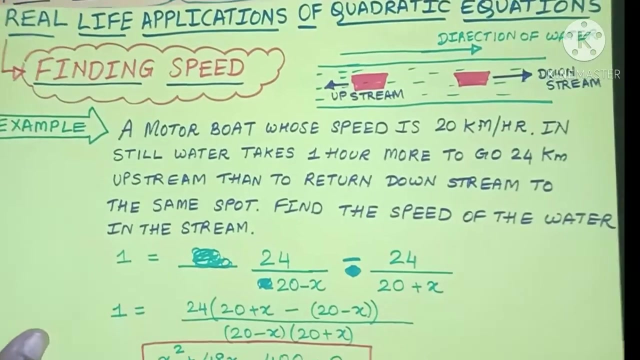 getting a quadratic equation friends. So this, when solved, will help us get the loss percent value. So quadratic equations is used a lot while calculating profit and loss. So in accounts and business profession also, quadratic equations is used. Now coming to the next Application of quadratic equations. well, it is used to find speed of objects. 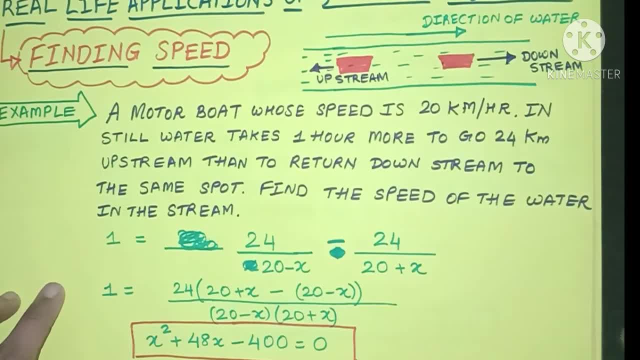 So, for example, here is an example to help you understand better. So suppose you have a stream and a motor boat is traveling, say, at a speed of 20 kilometer per hour in still water. So, friends, suppose the direction of the water in the stream is, say, this way: 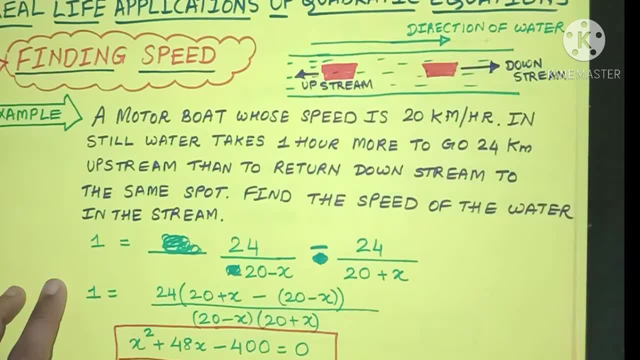 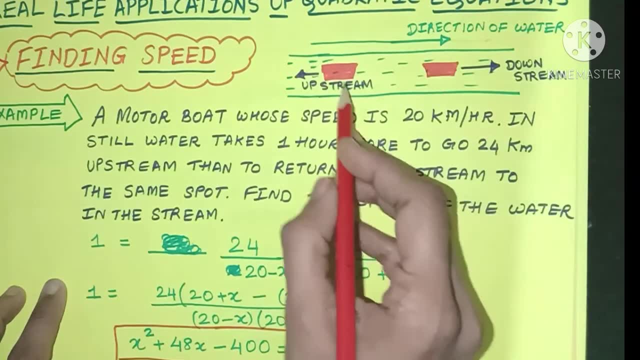 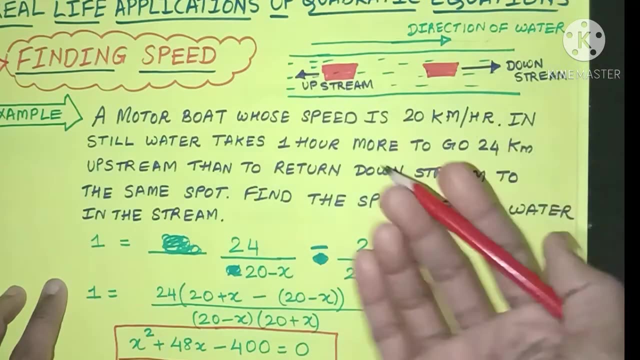 Then downstream means when the boat travels in the same direction as that of the water, And upstream is when the boat travels against the direction of water, that is, it is an opposite direction. So obviously when the boat is traveling upstream it will take more time. 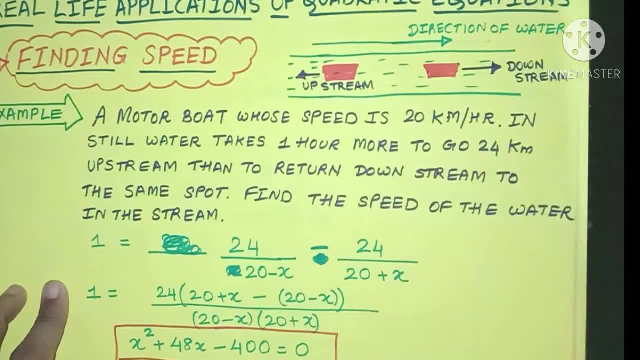 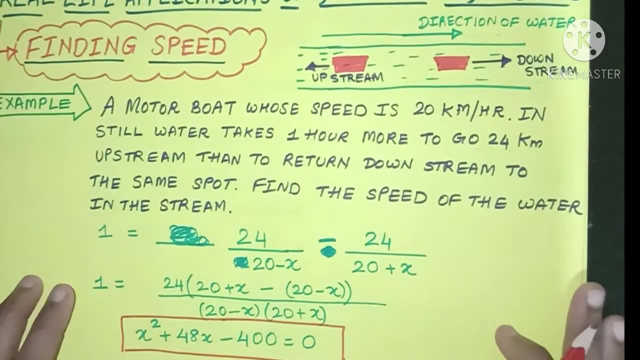 So suppose it is taking one hour more to go, you know, to a distance of 24 kilometers than when it is traveling downstream to cover the same distance. And you know we have to find the speed of the water in the stream. This is very much possible with the help of quadratic equations. 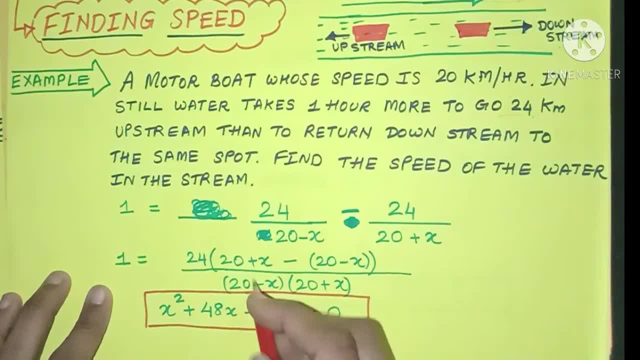 So you use the distance speed time formula. So the difference in the time is one hour and you have distance in the numerator and the speed in the denominator. So when you do this particular simplification again you will get a quadratic equation which, when solved, will give us the speed of the water in the stream. 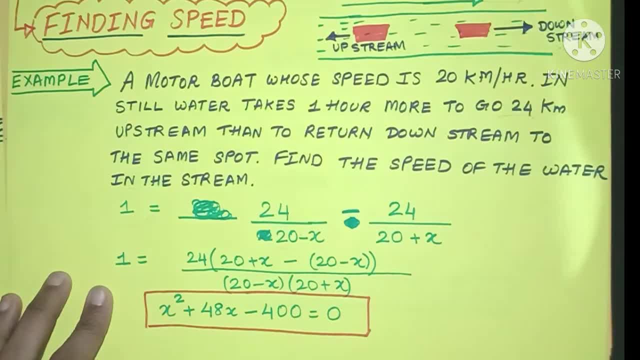 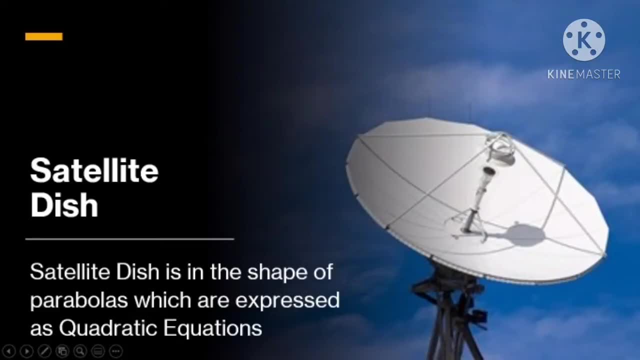 So you will see, friends, that quadratic equation is so important in finding such values. So, friends, quadratic equations are used in the design of satellite dishes, because satellite dish is in the shape of parabolas which are mathematically expressed as quadratic equations. So the knowledge of quadratic equations is very important while designing these satellite. 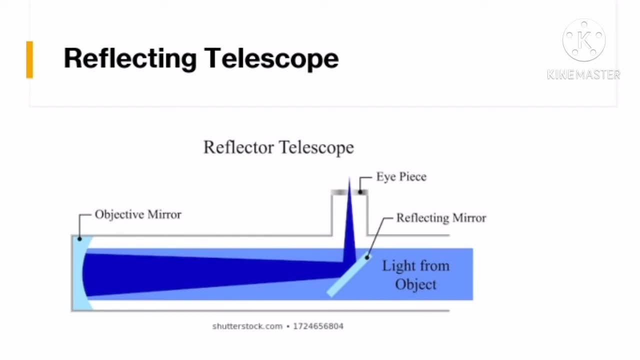 dishes. Friends, here is a reflecting telescope, and in a reflecting telescope, the primary mirror is the parabolic mirror, and to design this parabolic mirror you need knowledge of quadratic equations, Because it is in the shape of parabola, which is mathematically represented using quadratic. 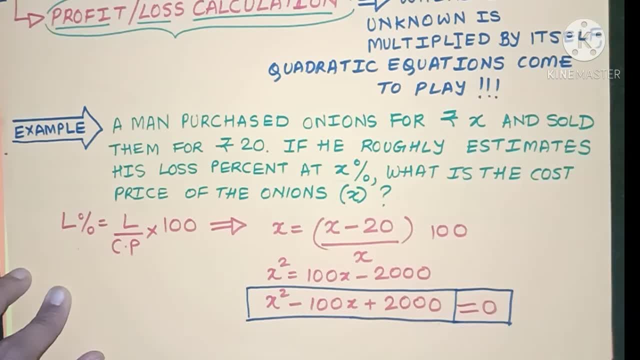 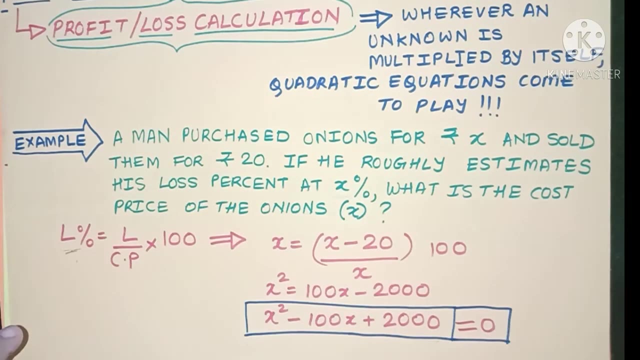 quadratic equation friends. So this, when solved, will help us get the loss percent value. So quadratic equations is used a lot while calculating profit and loss. So in accounts and business profession also quadratic equations is used. Now coming to the next application of quadratic equations. 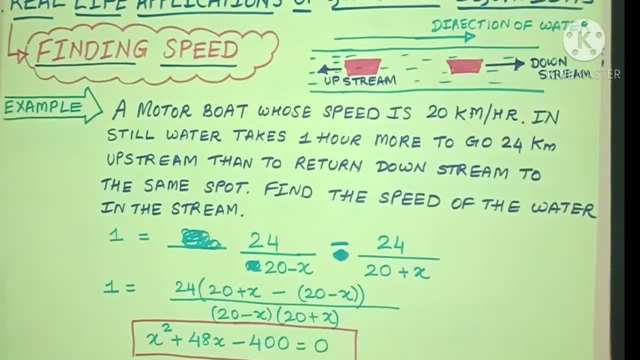 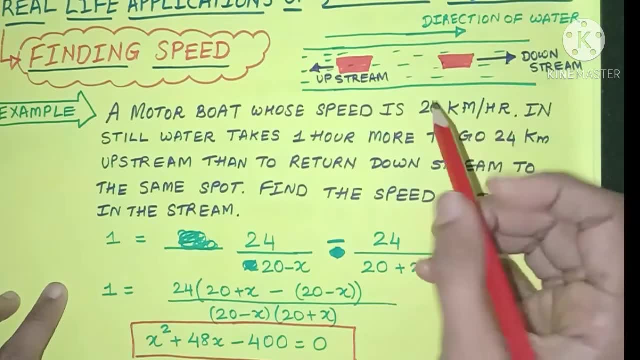 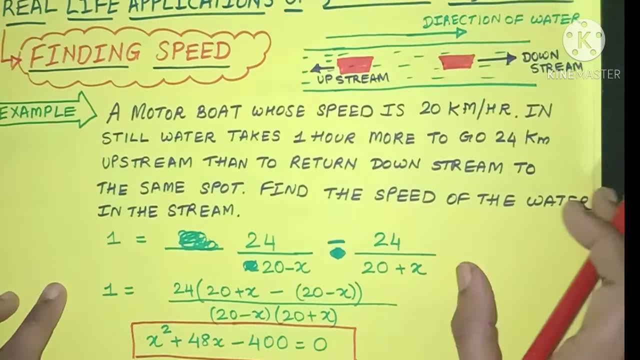 Well, it is used to find speed of objects. So, for example, here is an example to help you understand better. So suppose you have a stream and a motorboat is traveling, say, at a speed of 20 kilometer per hour in still water. So, friends, suppose the direction of the water in the stream is, say this: 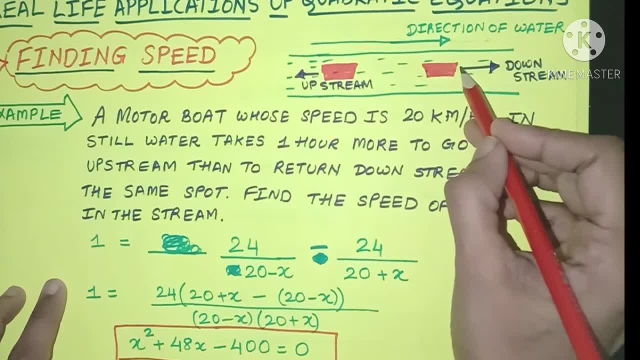 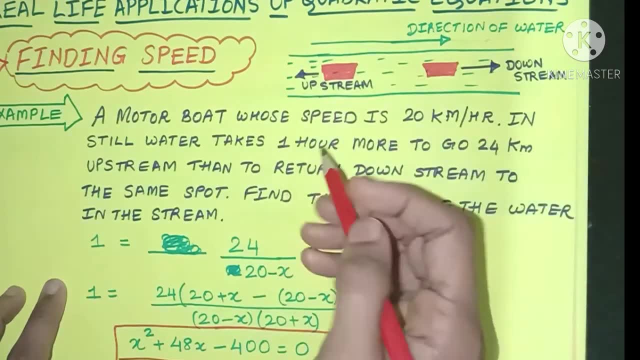 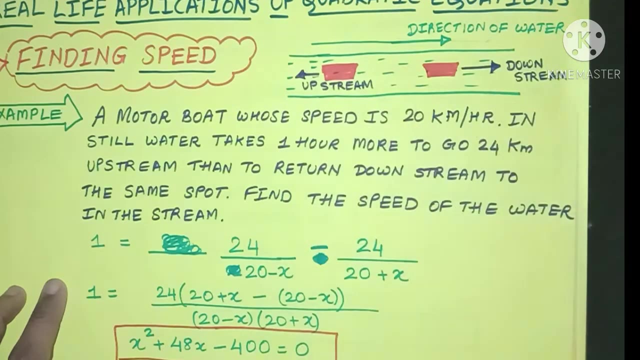 way, Then downstream means when the boat travels in the same direction as that of the water, and upstream is when the boat travels against the direction of water, that is, it is an opposite direction. So obviously when the boat is traveling upstream it will take more time. So suppose it is. 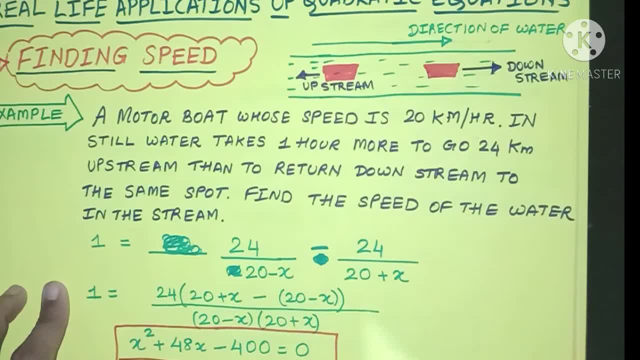 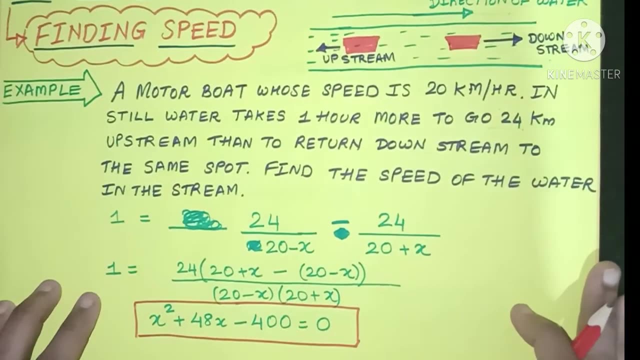 taking one hour more to go, you know, to a distance of 24 kilometers, than when it is traveling downstream to cover the same distance. and you know we have to find the speed of the water in the stream. This is very much possible with the help of quadratic equations, So let us see how this 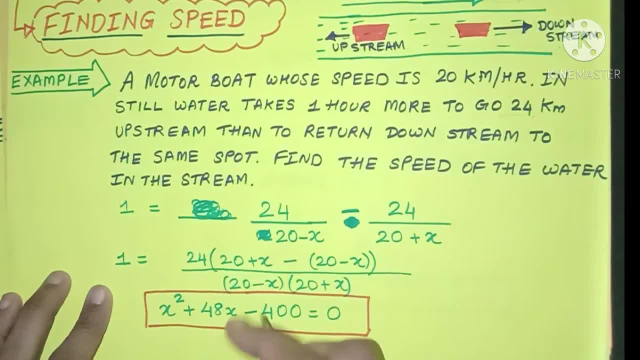 works. So you use the distance speed time formula. So the difference in the time is one hour and you have distance in the numerator and the speed in the denominator. So when you do this particular simplification, again you will get a quadratic equation which, when solved, will give us the speed. 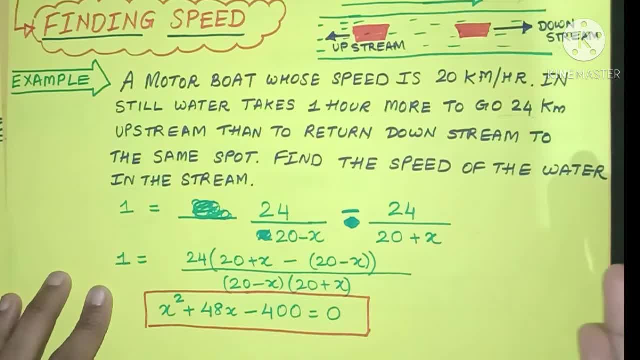 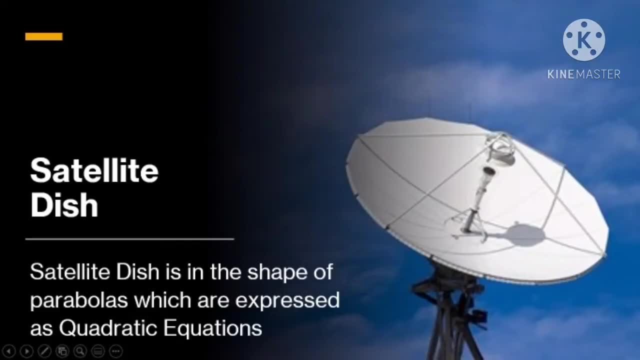 of the water in the stream. So you will see, friends, that quadratic equation is so important in finding such values. So, friends, quadratic equations are used in the design of satellite dishes, because satellite dish is in the shape of parabolas which are mathematically expressed as quadratic equations. So the knowledge, 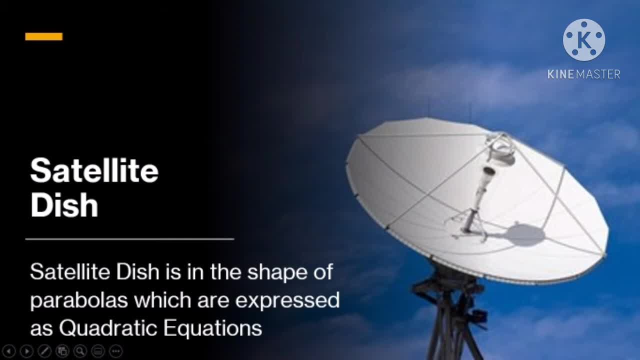 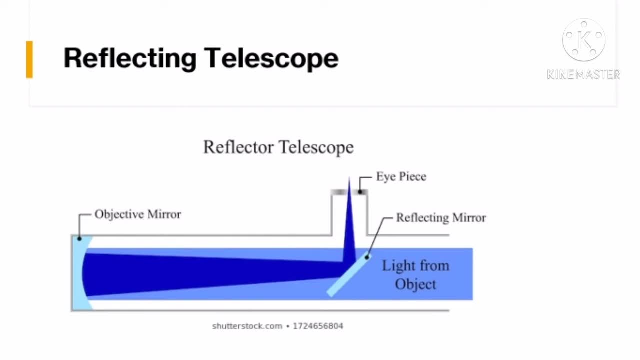 of quadratic equations is very important while designing these satellite dishes. Friends, here is a reflecting telescope, and in a reflecting telescope, the primary mirror is the parabolic mirror. and to design this parabolic mirror you need knowledge of quadratic equations, because it is in the shape of parabola, which is mathematically